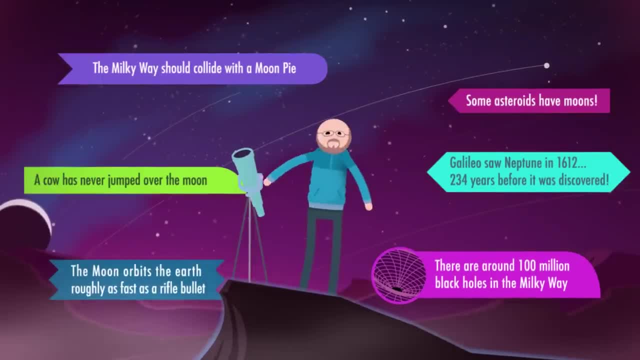 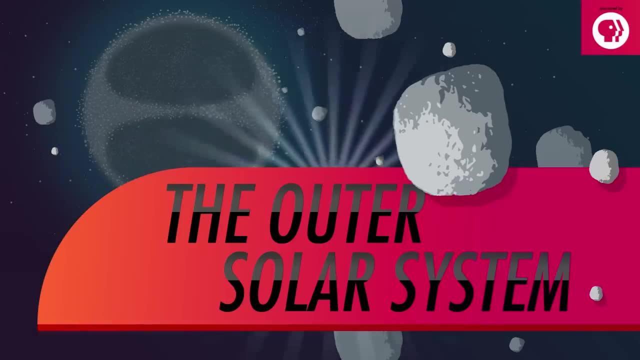 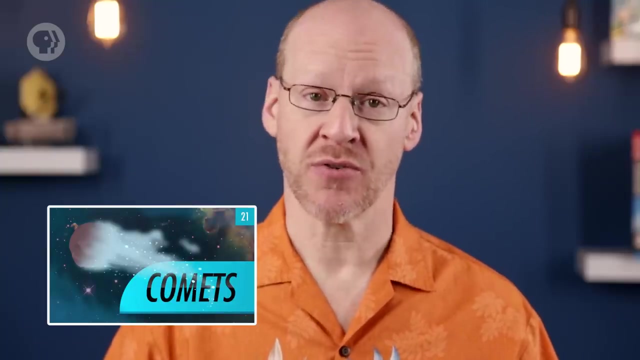 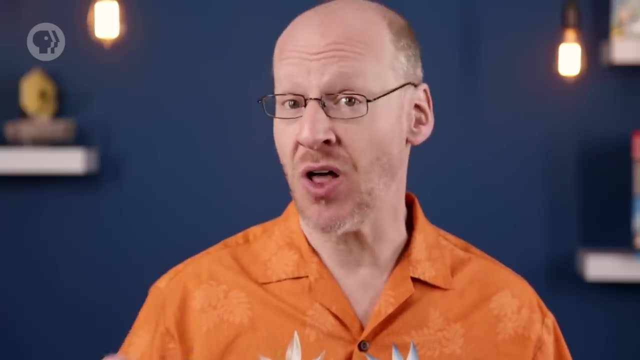 One giant leap for mankind. The empty space past Neptune isn't exactly… empty. In episode 21, I mentioned that comets come in two varieties: those with orbital periods of less than 200 years, which tend to orbit the Sun in the same plane as the planets, and those with longer periods, which have orbits tilted every which way. This is something of a problem. Comets lose material when they get near the Sun Over the course of millions of years. the Sun's orbit is tilted every which way. This is something of a problem. Comets lose material when they get near the Sun Over the course of millions of years. 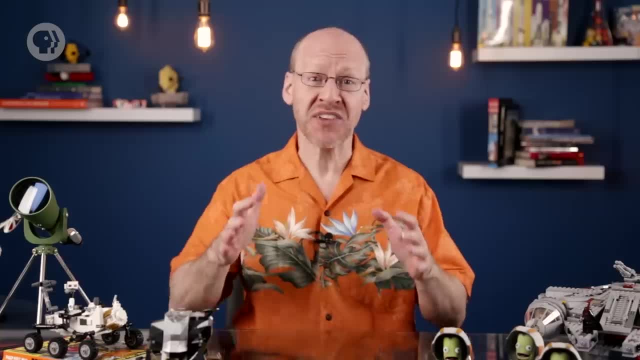 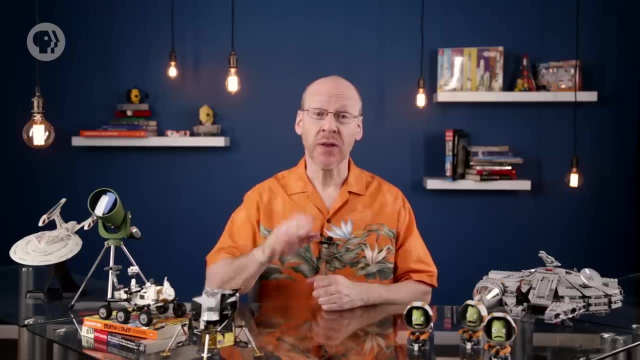 these comets should evaporate. And yet here we are, 4.56 billion years after the Solar System's birth, and comets still appear in our skies. So where are they coming from? To see, we'll have to turn the clock back a wee bit like. 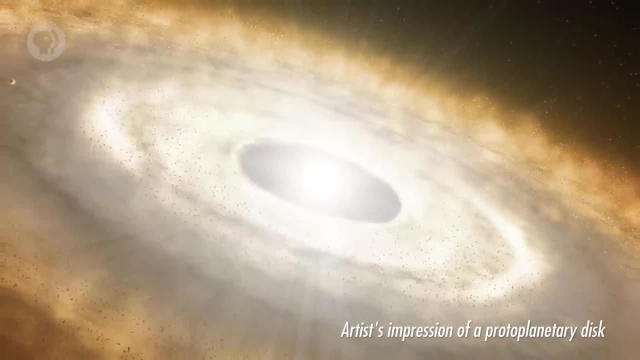 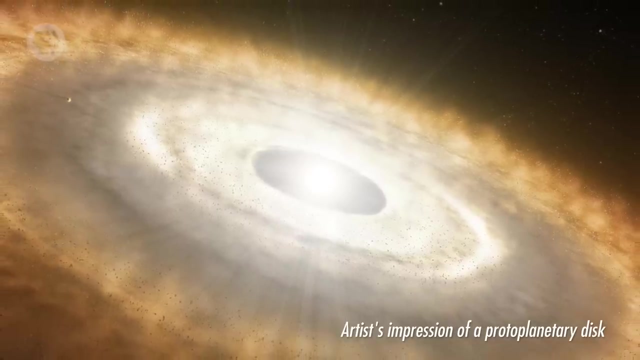 4.5 billion years. Behold our forming Solar System Coalescing out of a flat disk of material around the Sun. the inner planets were warmer, smaller and rocky, while the outer planets were in a region that was colder and grew huge Out there, in the chillier part of the Solar System. 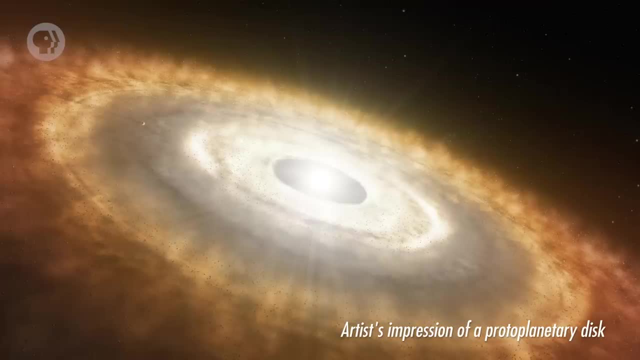 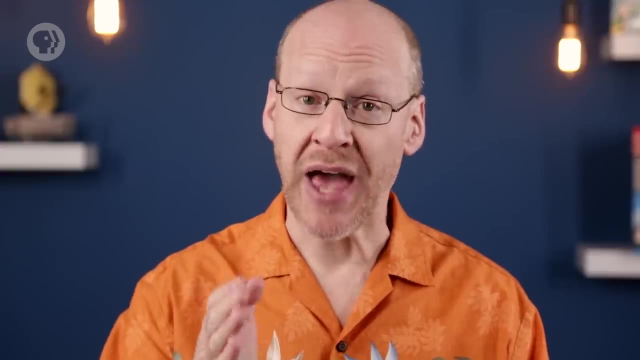 water came in the form of ice mixed in with dust and other stuff. These bits would collide and stick together, growing bigger. Some grew to hundreds of kilometers across. But there was a problem: Those outer planets. They had a lot of gravity and any chunk of 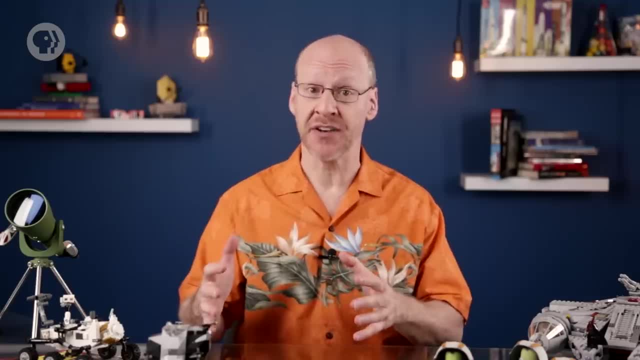 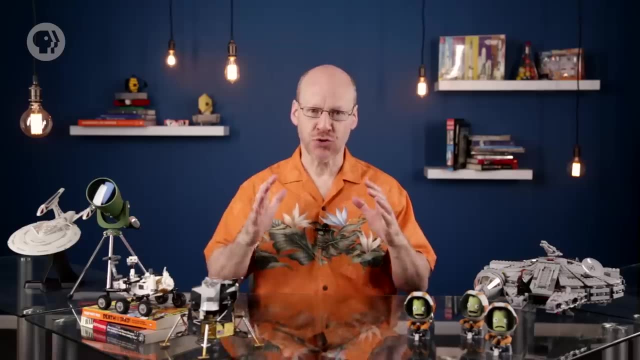 ice getting too close would either fall into the planet and get assimilated or get kicked into a different orbit. It could then plunge in toward the Sun or get flung out into deep space. Trillions upon trillions of such iceballs got tossed around by the planets, Even though they were small compared to the planets. they were still very small and they could still pull on the planets. They did have a little bit of mass and gravity, so every time the planet pulled hard on them, they also pulled a little bit on the planets too. It wasn't much per chunk, but after trillions of events. this adds up A current model of what happened, called the Nice model, after the city in France where it was proposed says that the overall effect of all these encounters was that Saturn, Uranus. 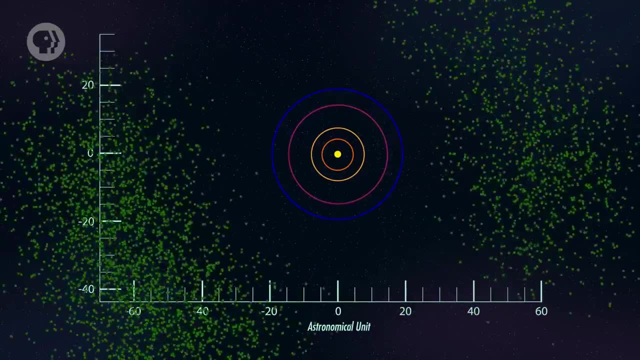 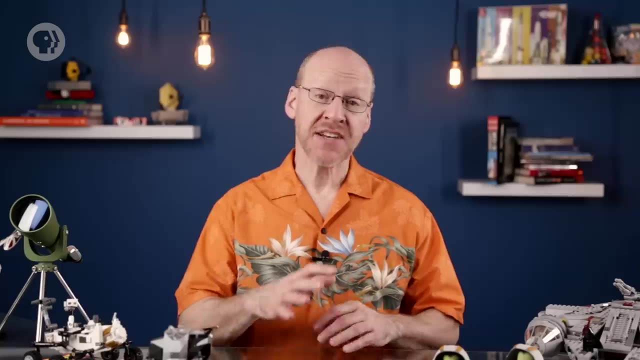 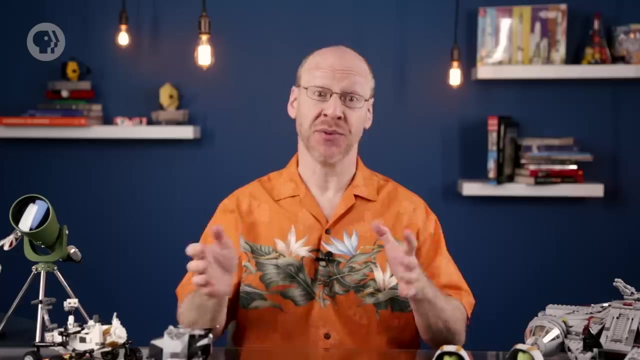 and Neptune slowly moved outward from the Sun. while Jupiter moved inward, Neptune would have the biggest volume of space where they lived. As Neptune migrated outward, close encounters with these chunks of ice flung lots of them into crazy orbits, highly elliptical and tilted with respect to the planets, Repeated more. 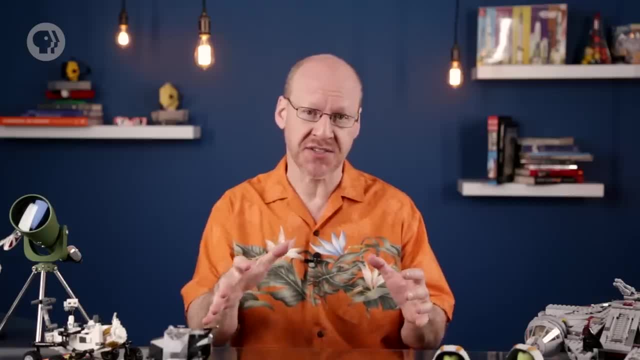 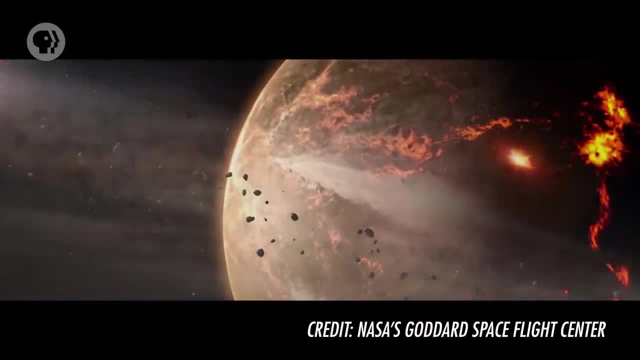 distant encounters tended to more slowly increase the sizes of the orbits of the iceballs too. We think that this shuffling around of the outer planets is what caused the late heavy bombardment, the intense shower of objects that came screaming down from the outer solar. 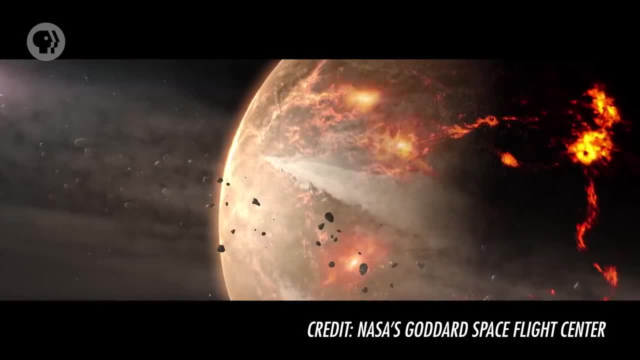 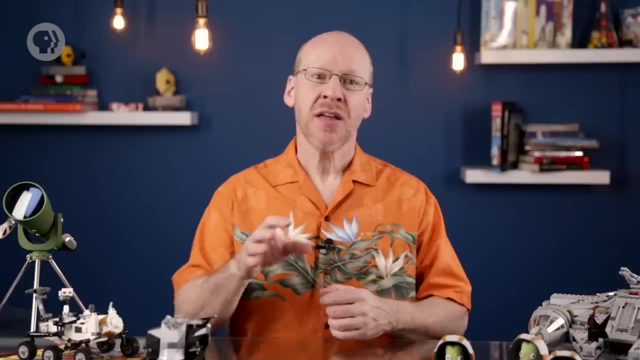 system, scarring planets and moons a few hundred million years after the planets themselves formed. It's not known for sure, but all the pieces fit together really well In the end. today, there are three rather distinct populations of these objects. One 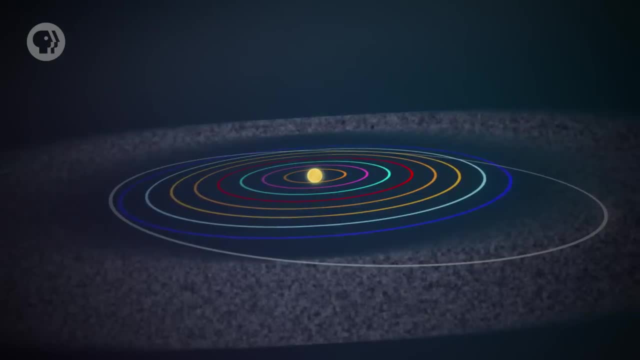 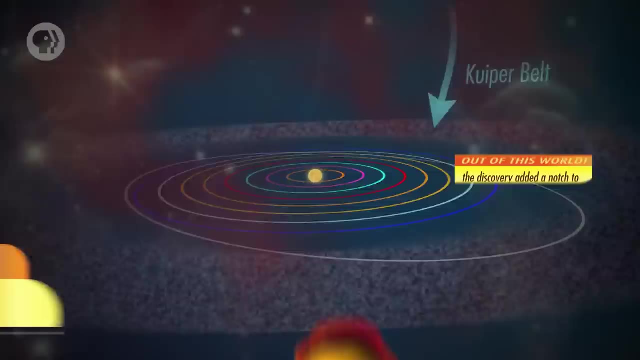 is a region shaped like a puffy disk or a donut, aligned with the plane of the planets. Icy objects there have stable orbits unaffected by Neptune. We call this the Kuiper belt, named after the Dutch astronomer Gerard Kuiper, one of many who initially speculated about 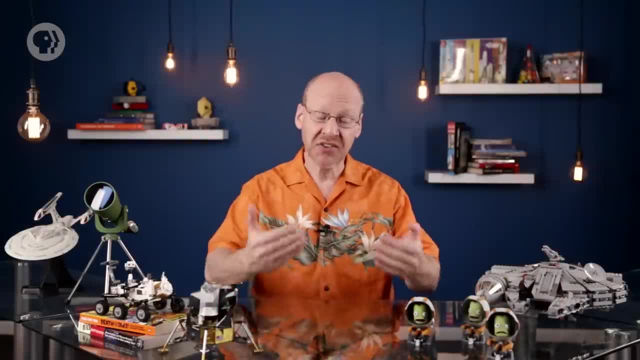 the existence of this region. The Kuiper belt starts more or less just outside Neptune's orbit, extending from about 4.5 million years ago. The Kuiper belt starts more or less just outside Neptune's orbit, extending from about 4.5. 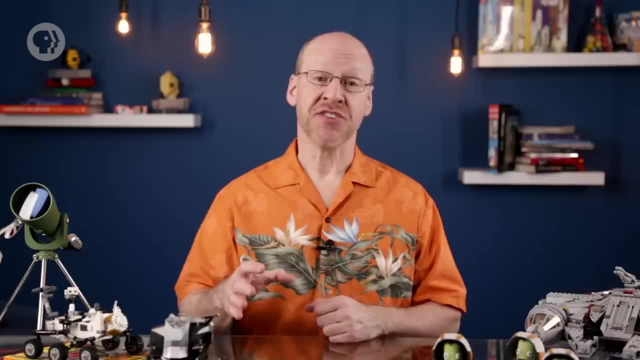 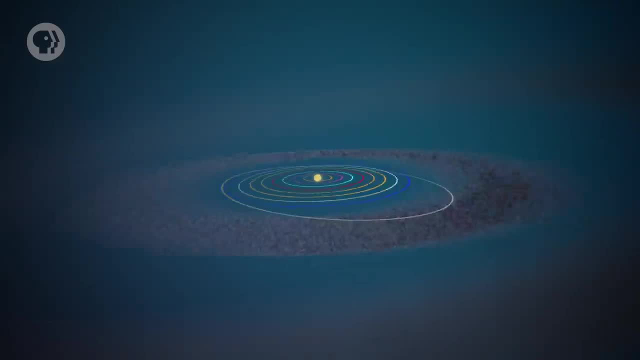 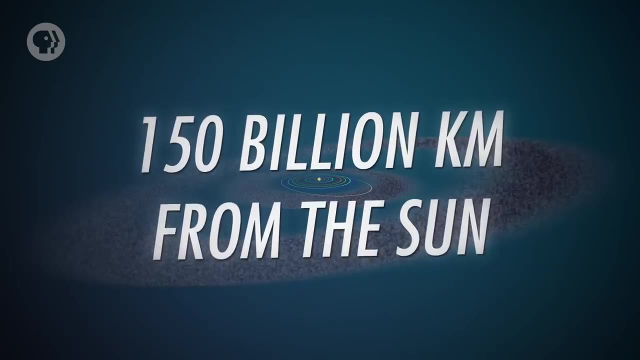 to 7.5 billion kilometers from the Sun. The second region is called the scattered disk. This is composed of the ice balls sent by Neptune into those weird highly tilted orbits. This overlaps the Kuiper belt on its inner edge and extends out to perhaps 150 billion kilometers from the Sun. That's. 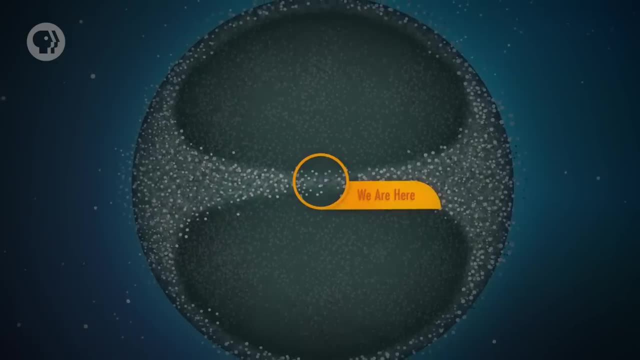 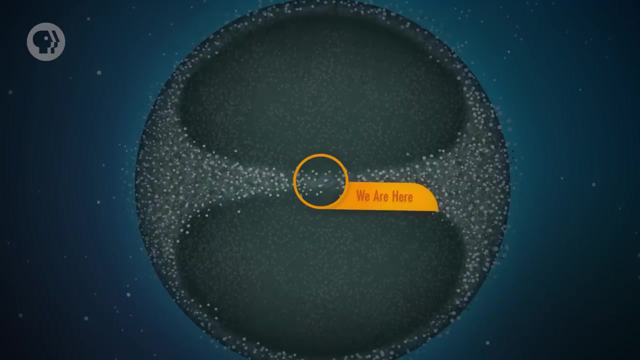 25 times farther out than Neptune. Finally, outside those two zones, there's a spherical cloud of icy objects which starts roughly 300 billion kilometers out, 70 times farther out than Neptune, A staggering 2,000 times the distance of the Earth from the Sun. And that's just where. 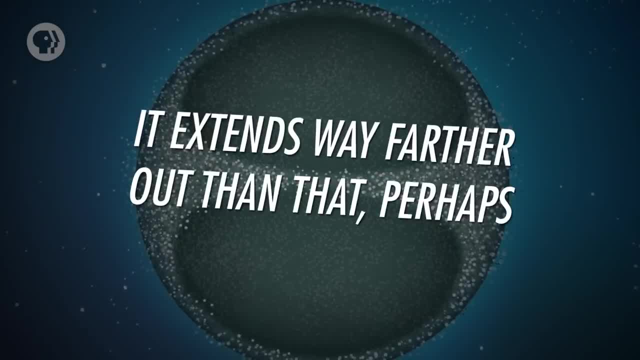 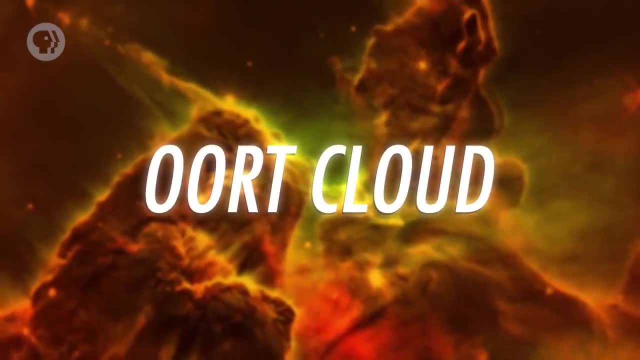 it starts, It extends way farther out than that, perhaps as much as a light-year, 10 trillion kilometers. This is called the Oort cloud after astronomer Jan Oort, who first proposed it. The Oort cloud is the origin of long-period comets, Since they orbit the Sun on a sphere. 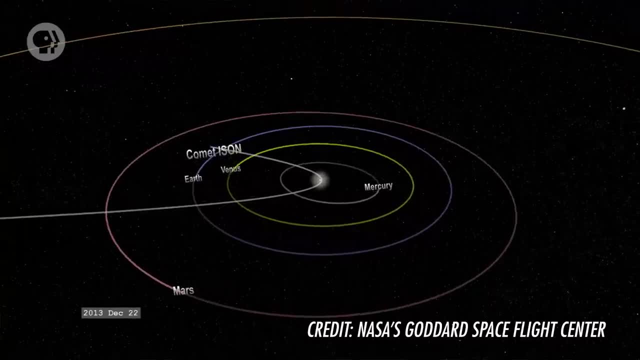 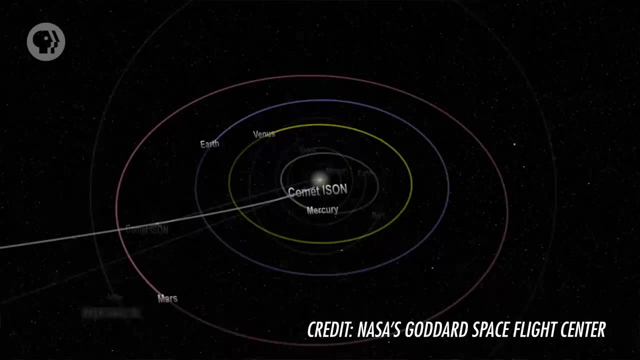 with no preferred orientation. they come in toward the inner solar system from random directions in the sky. Many newly discovered comets fall into this category. Their orbits can be extremely long. They start their fall from so far away. they swing around the Sun. 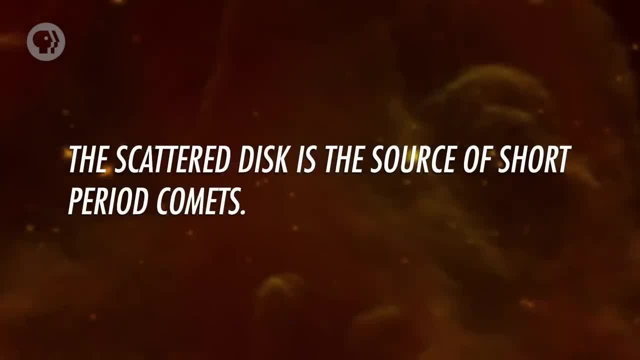 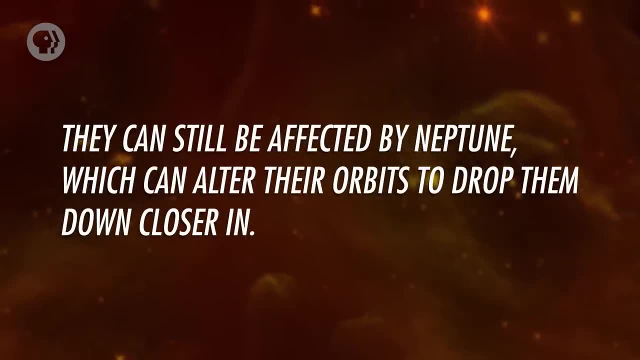 at nearly escape velocity and their orbits are close to being parabolic. The scattered disk is the source of short-period comets. They can still be affected by Neptune, which can alter their orbits to drop them down closer in. They can orbit the Sun on. 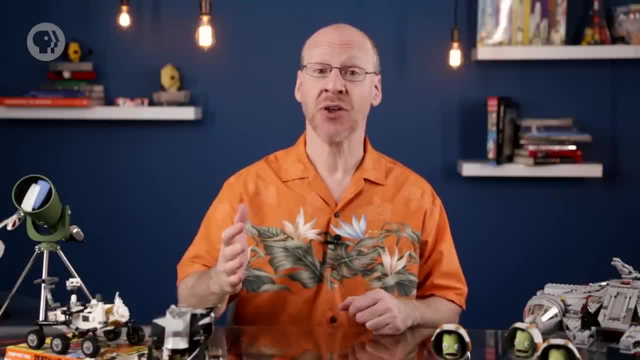 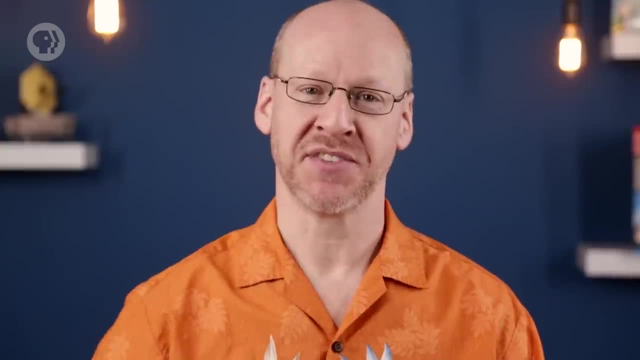 paths between Jupiter and Neptune, meaning eventually they'll have a close encounter with Jupiter. This can send them in closer to the Sun and they become short-period comets. Ta-da, That's how comets are made. So how do we know all this? 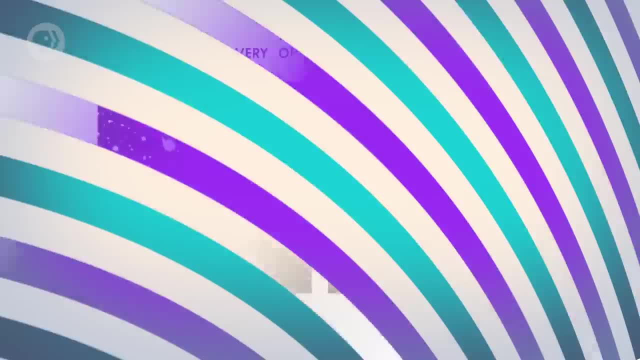 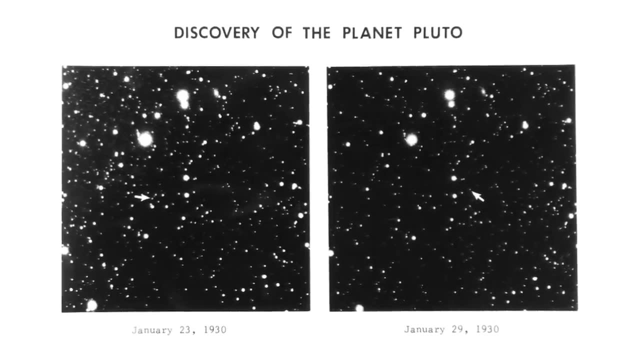 Well, until 1930, it was pretty much just conjecture. But then an American astronomer, Clyde Tombaugh, discovered the first Kuiper belt object, Pluto. Pluto orbits the Sun on an elliptical, mildly tilted path. Its orbit actually brings it closer to the Sun than 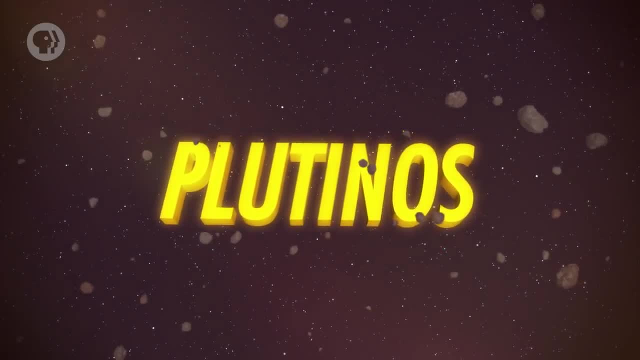 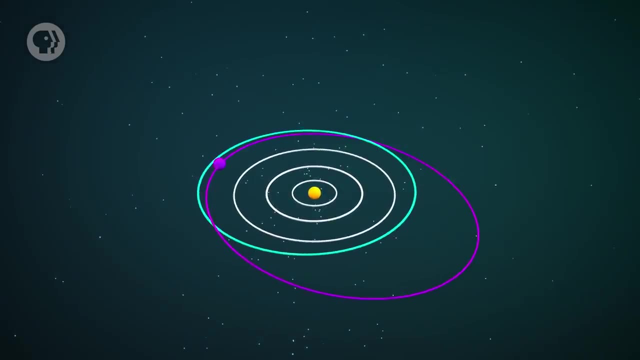 Neptune. So how come it never collides with the larger planet? Pluto's orbit crosses Neptune's more or less. Because the orbit is tilted, they never actually physically cross. When Pluto is at perihelion closest to the Sun, it's well above the plane of. 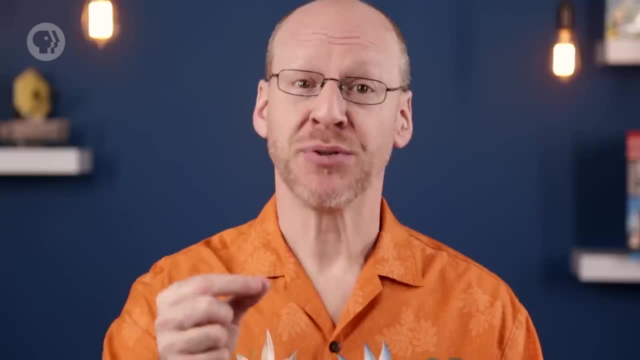 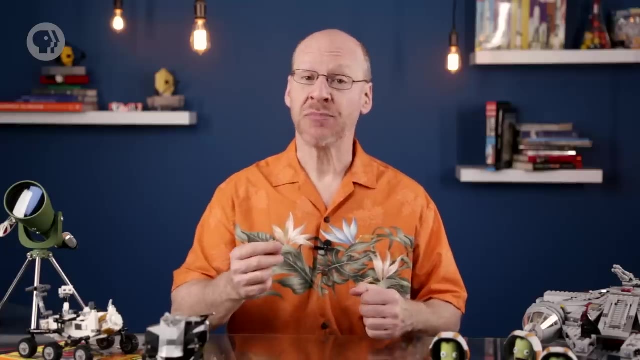 the solar system far from Neptune. Not only that, but Pluto orbits the Sun twice, for every three times Neptune does. Because of this, whenever Pluto is closest to the Sun, Neptune is always 90 degrees away in its orbit, That's many billions of kilometers distant, way too far to affect Pluto. 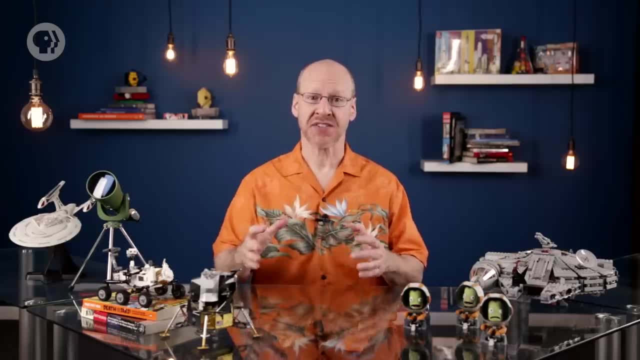 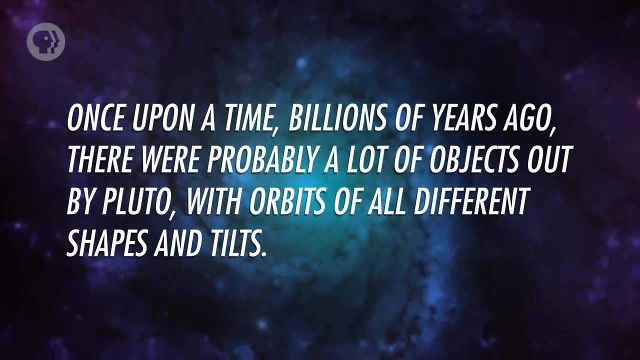 This is mostly coincidence. We've seen how orbital resonances can be forced by tides and by gravity, But in this case it's due to attrition. Once upon a time, billions of years ago, there were probably a lot of objects out by Pluto with orbits of all different. tilts, But the ones that got too close to Neptune got gravitationally tweaked into different orbits, turning them into comets or flinging them deeper into space. The only ones that could survive just happened to have orbits with that 3-to-2 or 2-to-1 resonance, with 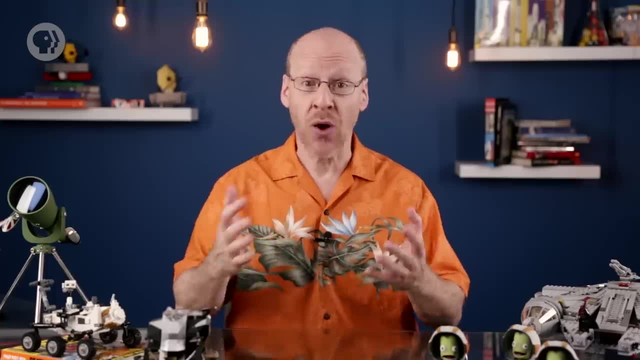 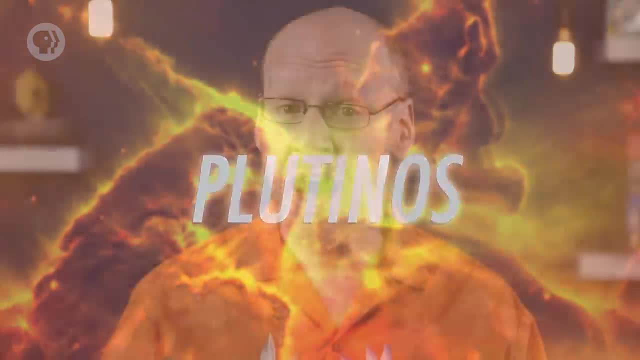 Neptune, keeping them far from Neptune's influence. Today those are the only kinds of objects we see with orbits near Neptune. We call these objects Plutinos. They're not really a separate class of object — they're still Kuiper belt objects — but a fun and 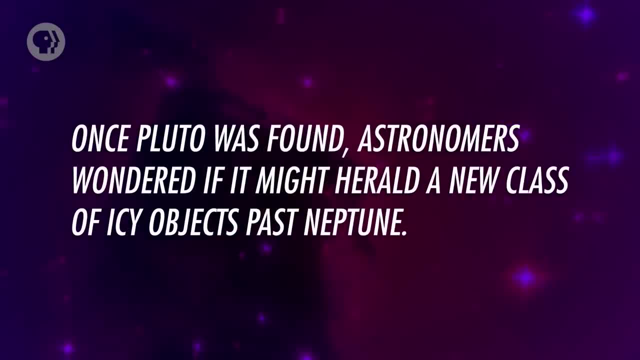 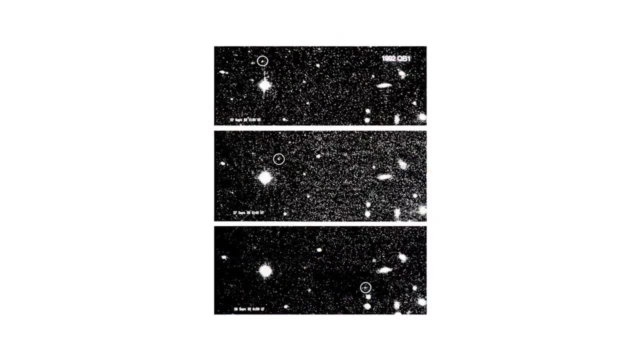 interesting subset of them, Pluto, was found. Astronomers wondered if it might herald a new class of icy objects past Neptune. However, it took more than six decades to find the next one, 1992. QB1 was discovered in 1992, and that opened a sort of gold rush of Kuiper belt discoveries. 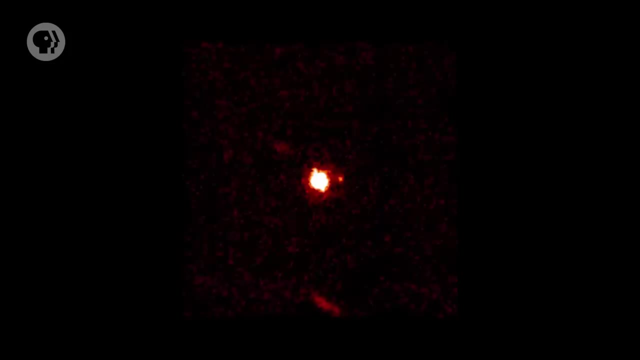 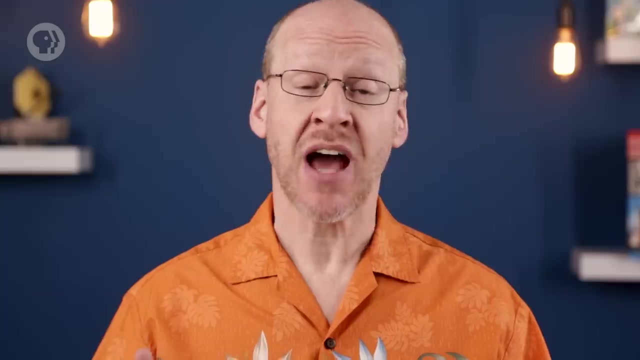 We now know of more than a thousand Kuiper belt objects. One called Eris is very close to Pluto's size and is more massive. It's probably rockier than icy Pluto. Pluto is an interesting object. A moon was discovered in 1978. Named Charon, it's actually about one-eighth the mass of Pluto itself. While Charon orbits Pluto, the moon has enough mass that it can be said that Pluto noticeably orbits Charon too. In reality, both circle around their mutual center of mass located between the two. Four more moons were discovered. 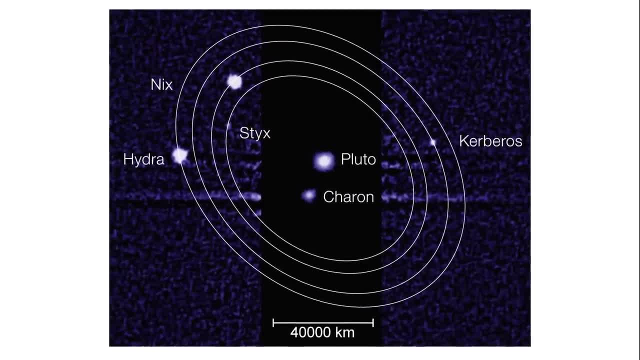 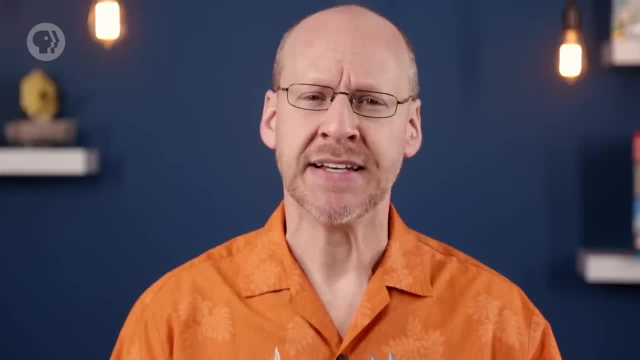 in Hubble images of Pluto in 2005 and 2012.. There may be more. Pluto is so small and distant that we don't know much about it, But that may be about to change. And now I have to admit to being in a tough spot As I record this episode. I'm going 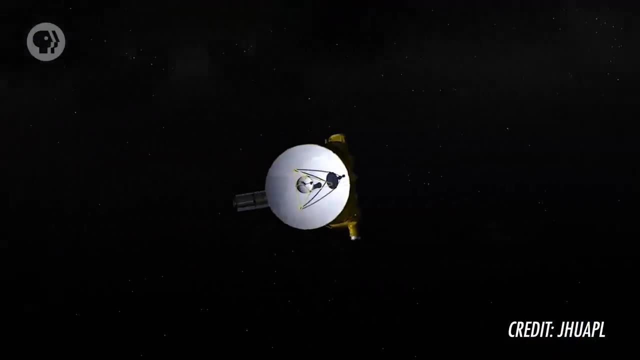 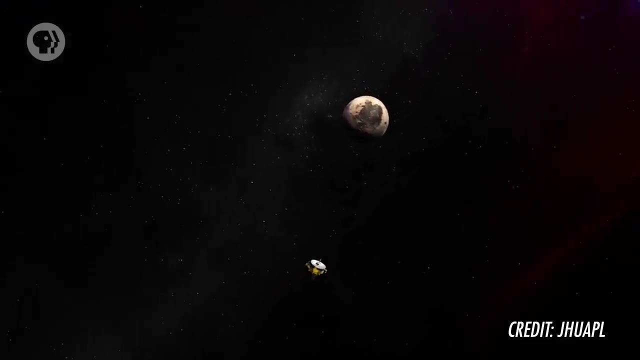 to tell you that in this episode of Crash Course, a space probe called New Horizons is heading toward Pluto. It'll fly by the tiny world in July 2015.. There's no doubt our view of Pluto will change. There may be more moons discovered. 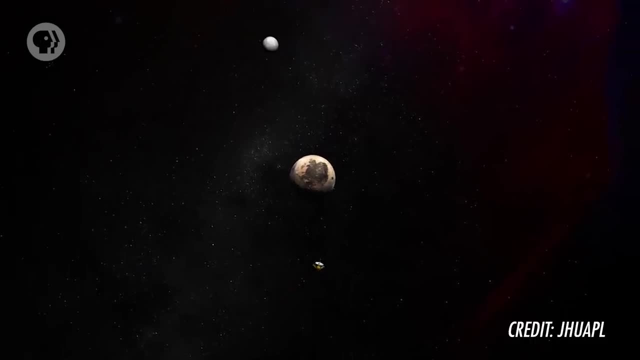 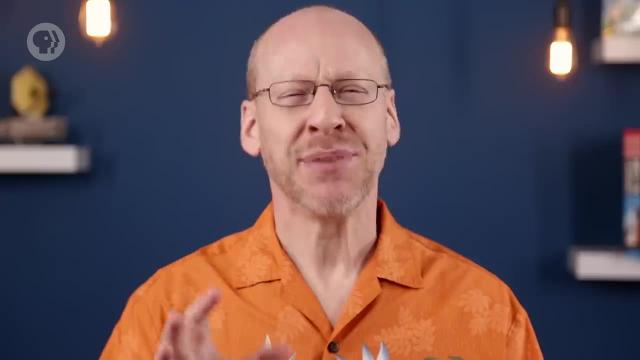 we'll see surface features for the first time and much more. But right now I can't tell you about any of that because we don't know yet. So I think the best thing to do is leave little Pluto alone for now. But there is a point I want to bring up. Pluto was found in 1930, long before any other Kuiper. 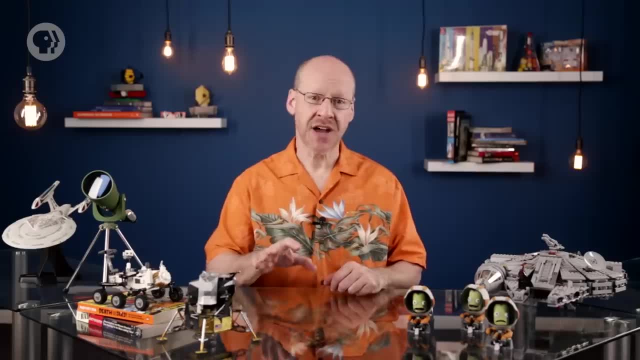 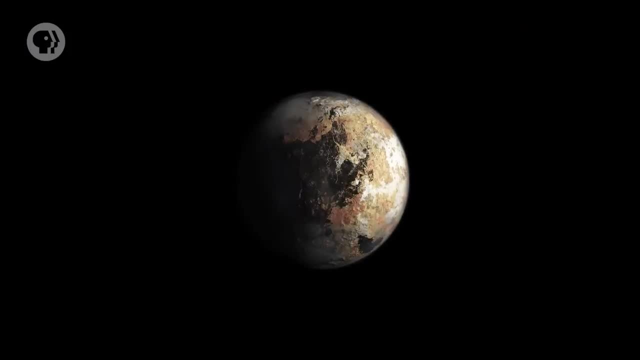 belt object because it's much brighter than any other. When it was discovered, it was thought to be about the size of Earth, But over the years, better observations showed it to be far smaller than first thought. In fact it's smaller. 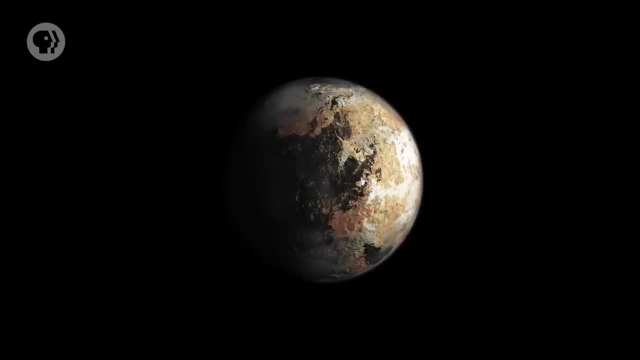 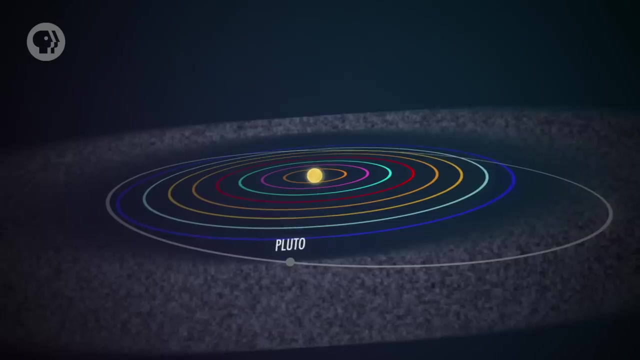 than Earth's moon. Its surface is unusually reflective, shiny, making it look much bigger than it seems. Most other Kuiper belt denizens are far less reflective and so are far fainter. If Pluto is king of the Kuiper belt objects, it has a lot of loyal subjects. We think the 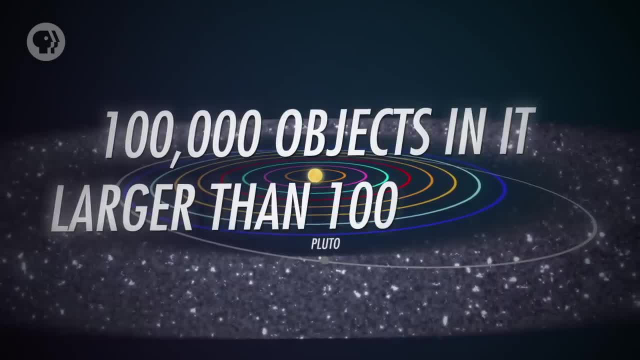 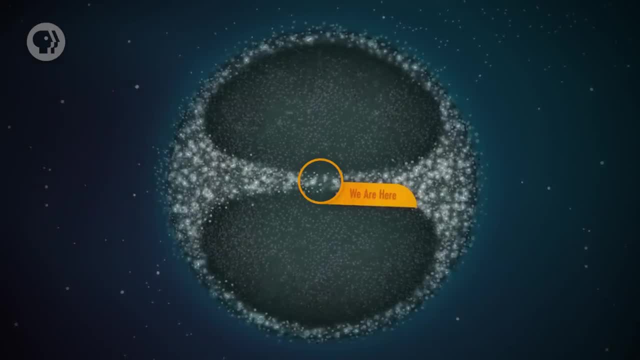 Kuiper belt may have 100,000 objects in it larger than 100 kilometers wide. If that sounds like a lot, get this. The Oort cloud surrounding the solar system may have trillions of icy bodies in it- Trillions. While we know lots of Kuiper belt objects we don't know of. any Oort cloud objects for sure. Two very interesting bodies have been found: Sedna and VP113.. Sedna's orbit takes it an incredible 140 billion kilometers from the Sun, while VP113 gets about half that far out. Both are on very elliptical orbits. Neither, however, gets close to Neptune, so it's not at all close. It's not at all clear how they got where they are. They may be Oort cloud objects that were disturbed by passing stars long ago, dropping them closer in to the Sun, But no one knows Yet. 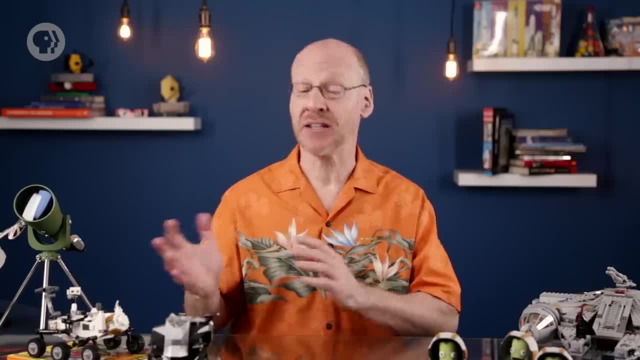 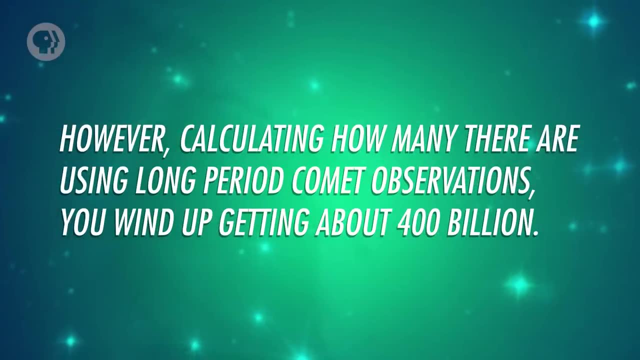 Speaking of which, we can calculate how many Oort cloud objects there should be left over from the formation of the solar system, and it's about 6 billion. However, calculating how many there are using long-period comet observations, you wind up getting about 400. 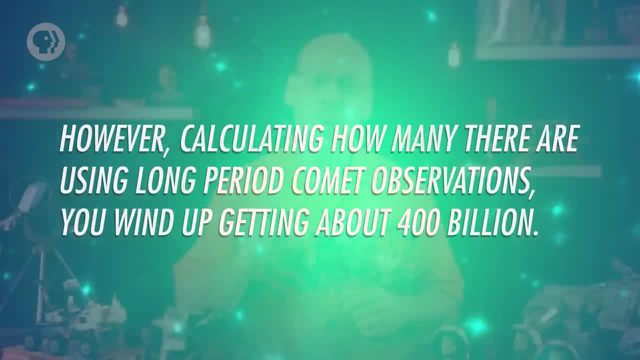 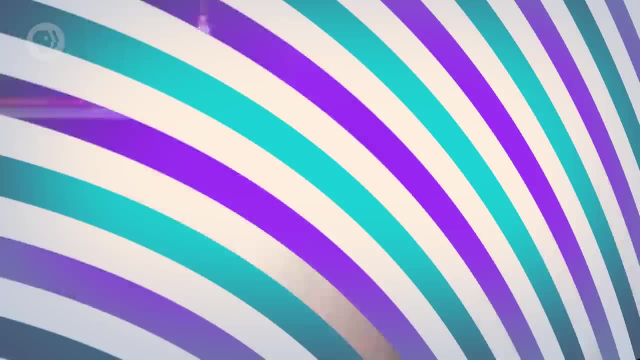 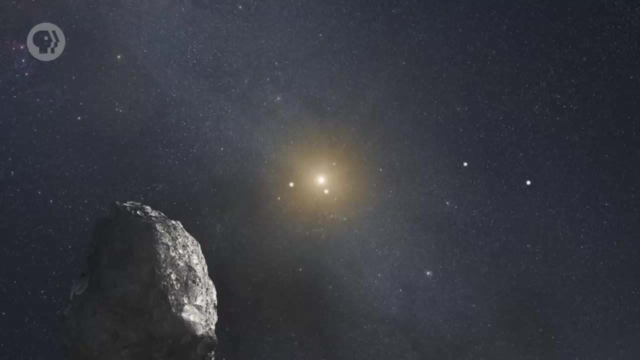 billion. That's a big discrepancy. Now get this To solve. this discrepancy is that the Sun has stolen comets from other stars. Seriously, Comets should form wherever stars do, and sometimes the Sun passes near other stars. When we see a long-period comet gracing our skies, could we be seeing an object from an? 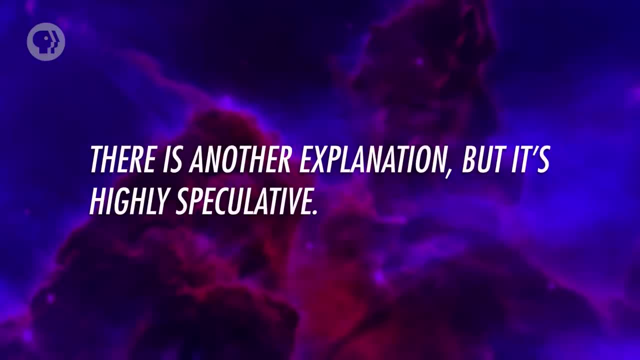 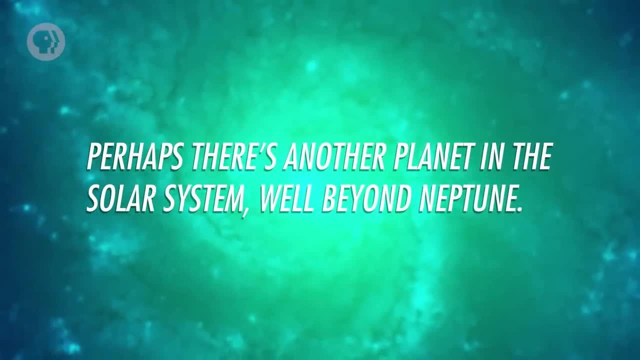 alien solar system. Maybe There is another explanation, but it's highly speculative. Perhaps there's another planet in the solar system well beyond Neptune? It's possible. Some very preliminary studies have shown that some long-period comets aren't comet-able.